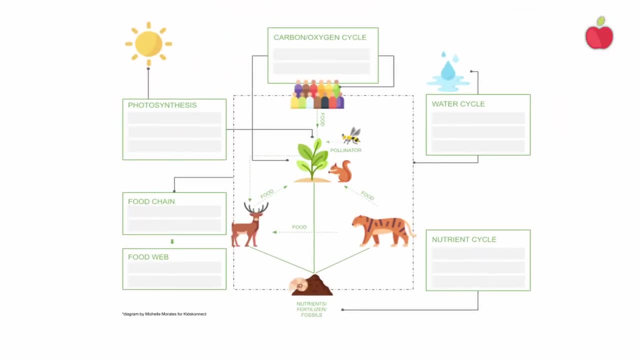 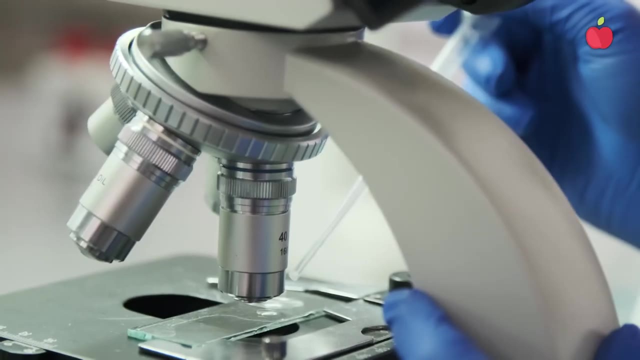 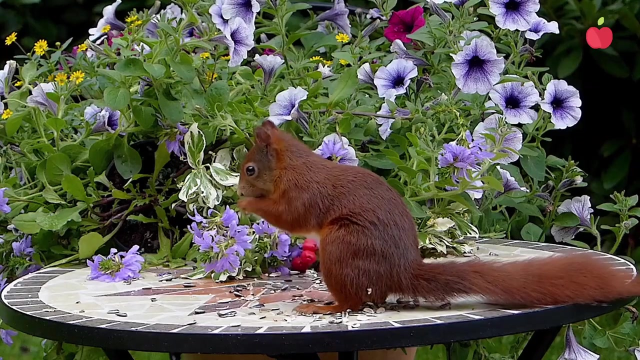 we humans are part of an ecosystem. Ecosystems are amazing communities of organisms creating a delicate web of life. Each component is crucial in maintaining balance, From the tiniest microbes to the largest predators. For example, plants convert sunlight into energy through photosynthesis. 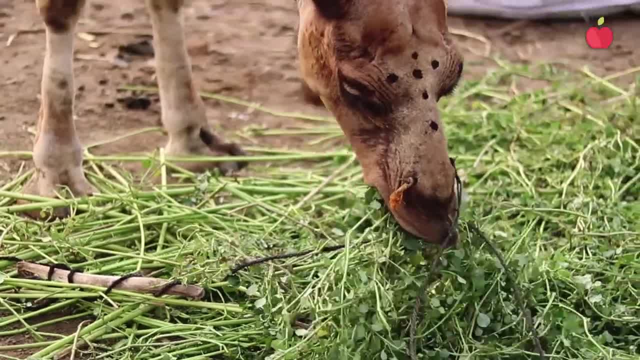 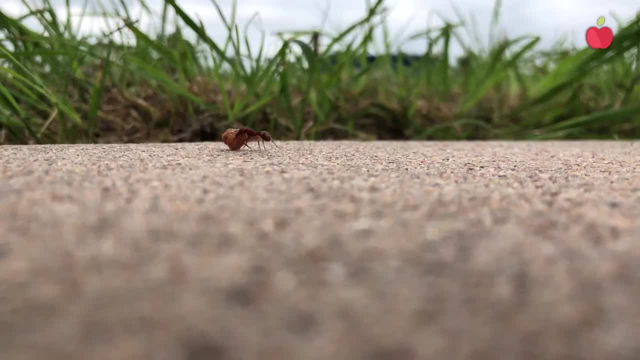 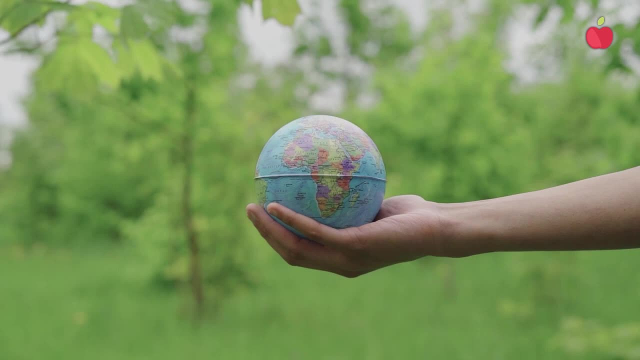 providing food and oxygen for other organisms. Herbivores then feed on plants. Carnivores hunt herbivores, And decomposers break down dead organic matter, recycling nutrients back into the ecosystem. There are many types of ecosystems found across our planet, each with unique characteristics and species compositions. Let's look closer at. 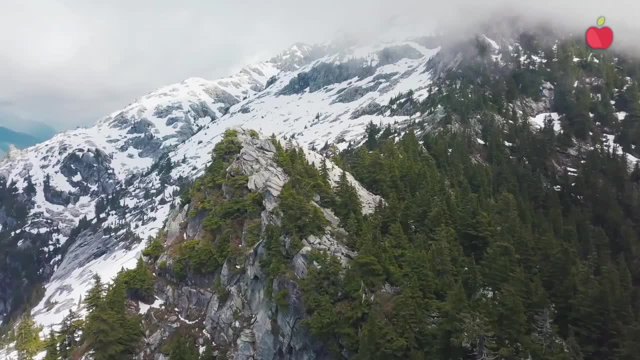 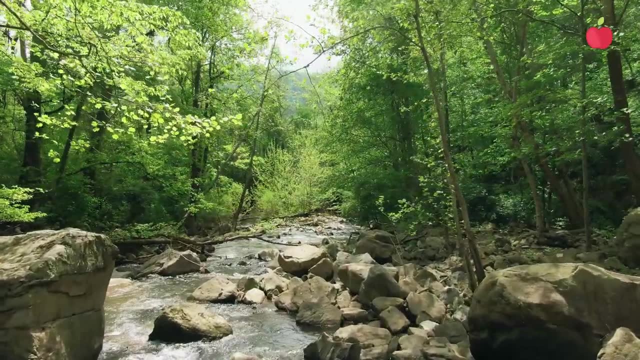 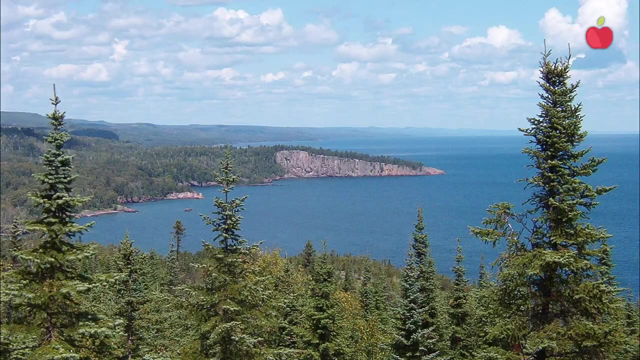 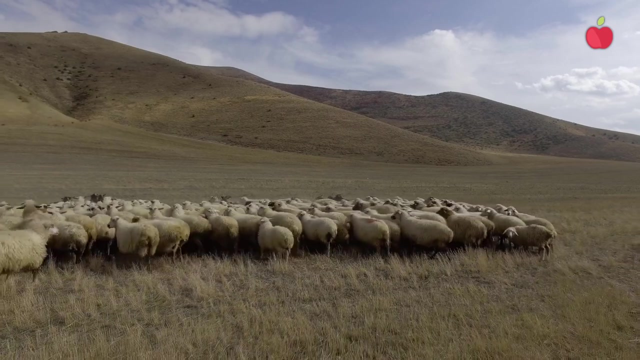 terrestrial, aquatic, polar, mountain and urban ecosystems. Our first stop takes us deep into terrestrial ecosystems, including forests, grasslands and deserts. Forest ecosystems include tropical, temperate and boreal forests characterized by diverse tree species and a dense canopy. Grassland ecosystems are found in areas with moderate rainfall. and are dominated by grasses supporting grazing animals like bison, antelope and zebra. Lastly, desert ecosystems are arid regions with sparse vegetation that's adapted to extreme temperatures and water scarcity. Cacti and reptiles are common desert inhabitants. 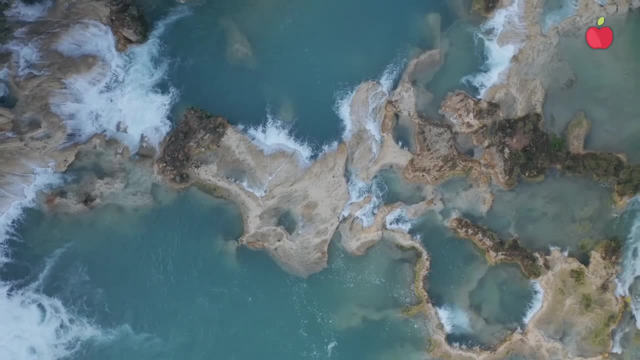 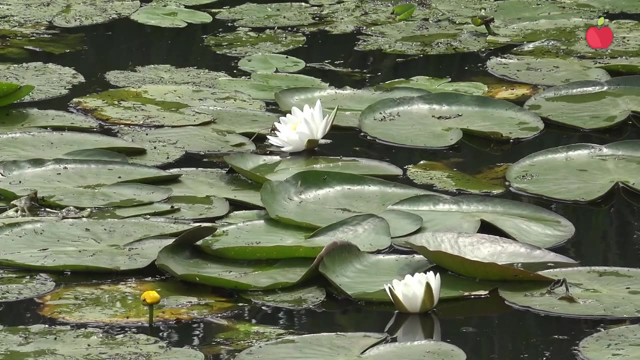 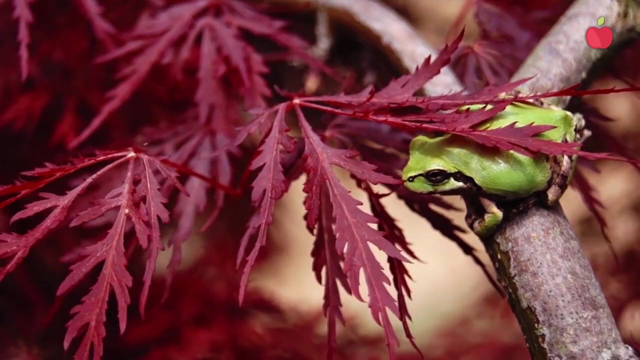 as well as marine ecosystems. Now let's plunge into aquatic ecosystems, including freshwater and marine ecosystems. Freshwater includes rivers, lakes, ponds and wetlands. They are home to fish, amphibians, aquatic plants and diverse microorganisms. Marine ecosystems cover vast. oceans, including coral reefs, estuaries and open ocean habitats, which support a rich array of marine life, including fish, marine mammals and marine animals. In addition, there are many marine ecosystems that cover vast oceans, including coral reefs, estuaries and open ocean habitats. 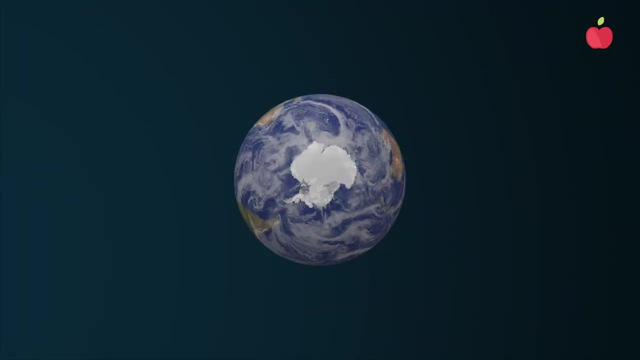 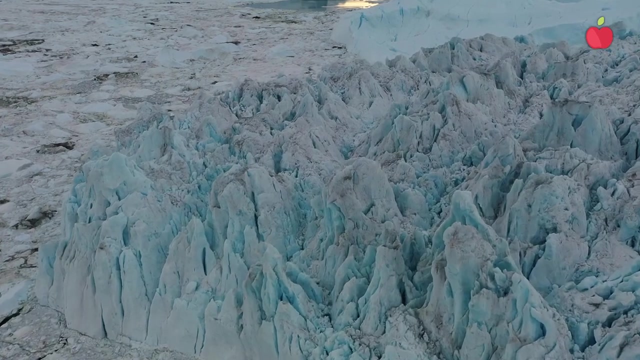 including marine animals and coral species. Now let's journey to the Arctic and Antarctic regions characterized by frigid temperatures and snowy landscapes. Polar ecosystems are home to specialized species like polar bears, penguins and seals, adapted to survive the cold. Next up mountain ecosystems are high-altitude areas characterized by cold temperatures, thin air and diverse flora and fauna, including alpine plants and elusive mountain-dwelling animals. Next up mountain ecosystems are high-altitude areas characterized by cold. 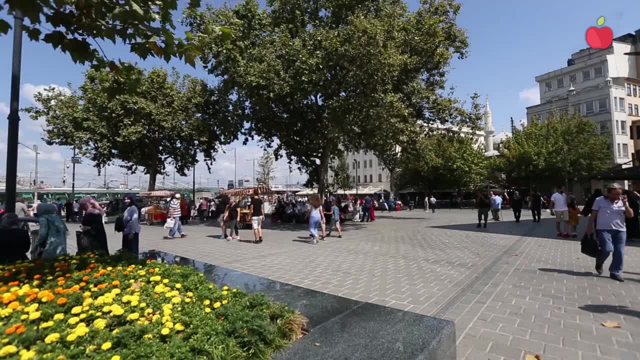 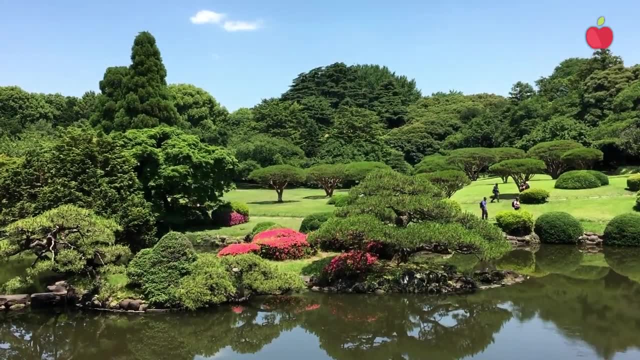 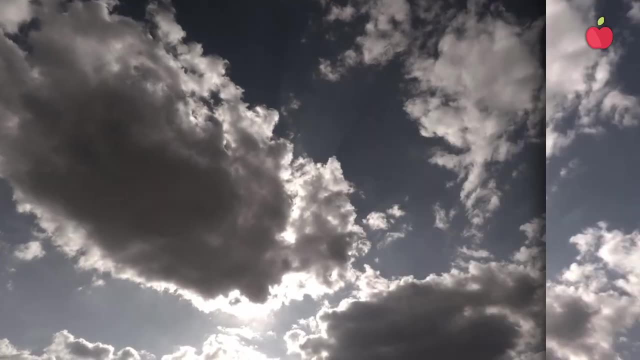 Meanwhile, the unique ecosystem shaped by human activities is called an urban ecosystem. Urban areas with parks, gardens and green spaces within cities provide habitats for birds, insects and plants, contributing to urban biodiversity. Ecosystems also provide essential human services such as regulating climate, purifying air. 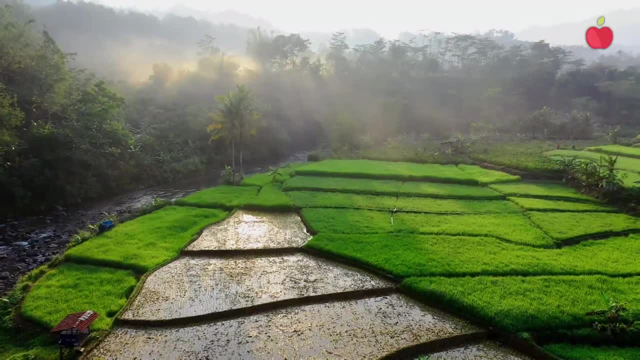 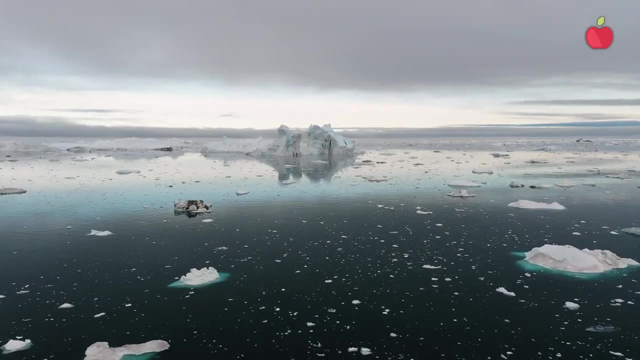 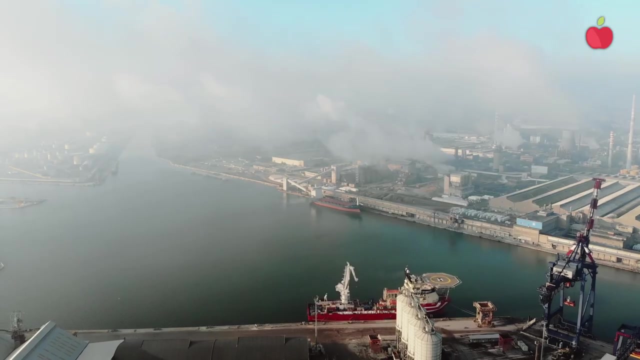 and water, pollinating crops, controlling pests and providing food, medicine and raw materials. But the dynamics of ecosystems have changed rapidly in a few centuries due to climate change and human activities like deforestation, pollution and habitat destruction.